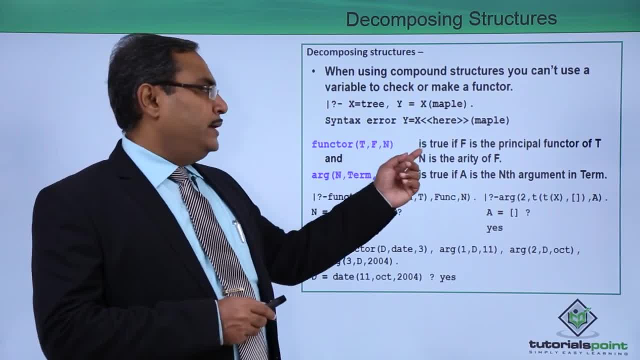 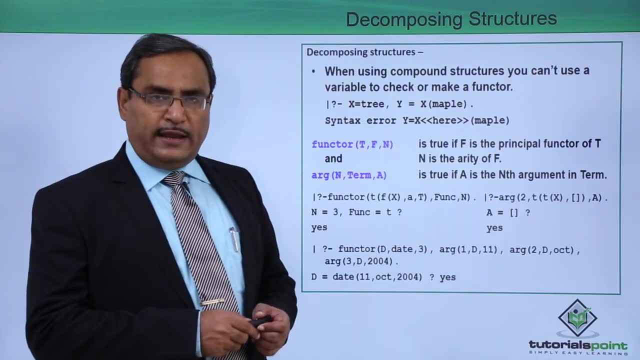 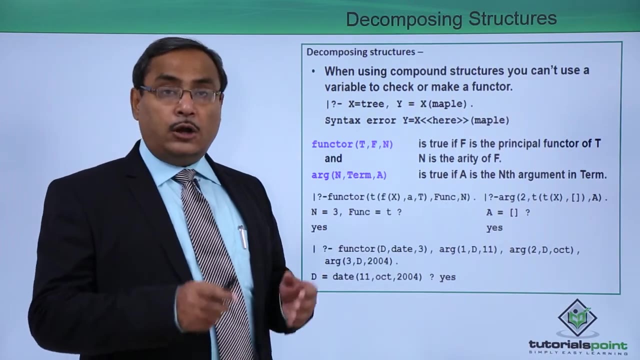 inbuilt predicate in prologue. Now, what is the purpose? It is true, if f is the principal functor of t and n is the addity of f, You might be asking me: what is addity? Addity means number of attributes, Addity means number of arguments. So what is the principal functor? So I think. 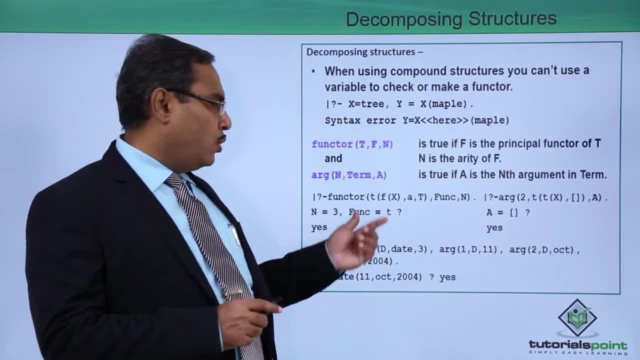 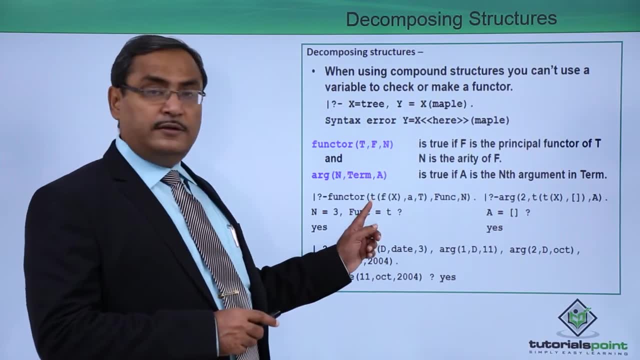 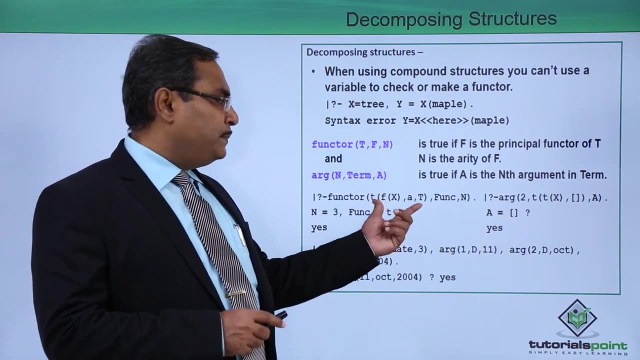 for the better understanding, let us go through one example: See functor. So here t is represented by this one. So here this is my functor name and three arguments are there. So this f will be taking the principal functor name, So t it will be taking. functor will be be t and this: 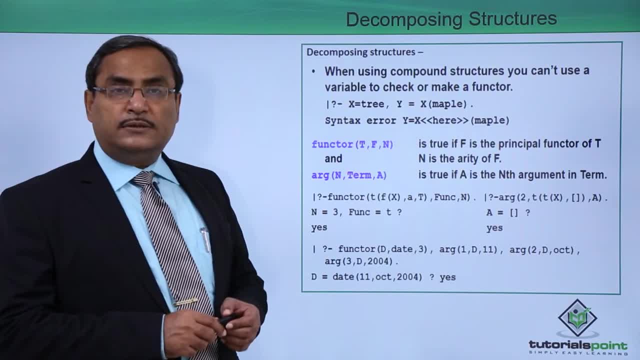 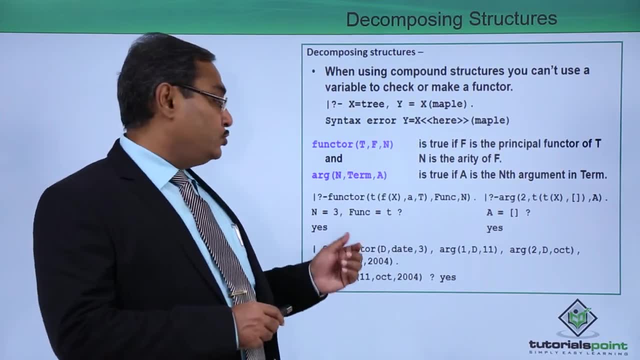 if n will be denoting the addity of the functor. What is the addity? How many arguments are there? One, two, three. So n will be initialized by three. So it will come like this: n is equal to three and funct is equal to principal functor name. Here it is t. So that is why. 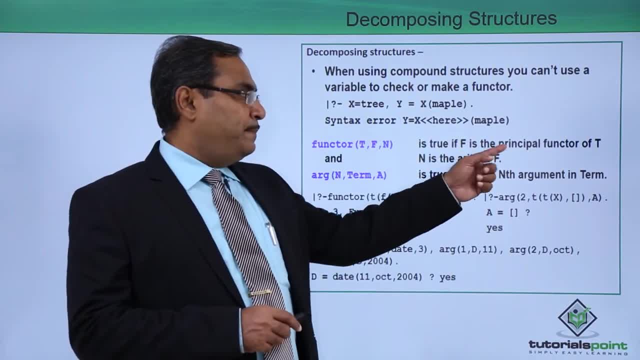 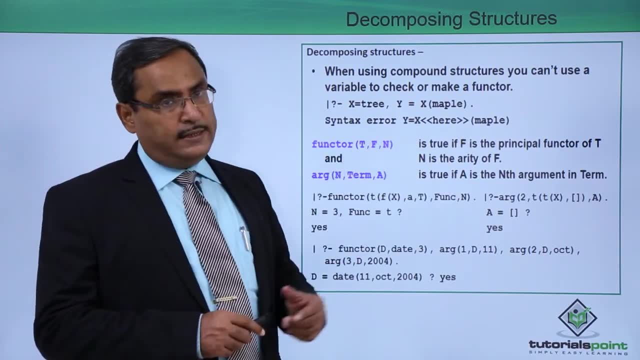 it has been written as is true. if f is the principal functor of t, n is the addity of f. So in this way we have represented this one. So let us go for d. So we have represented, just because. very well, So you can see what is the next step. 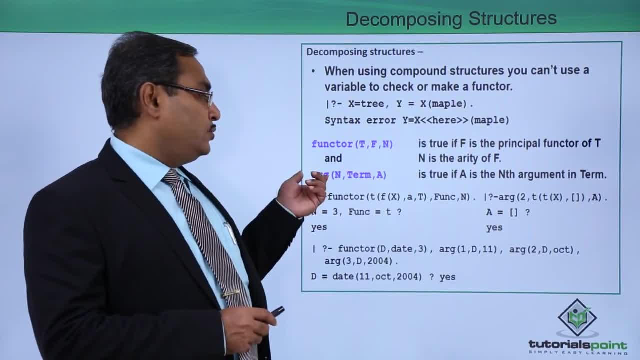 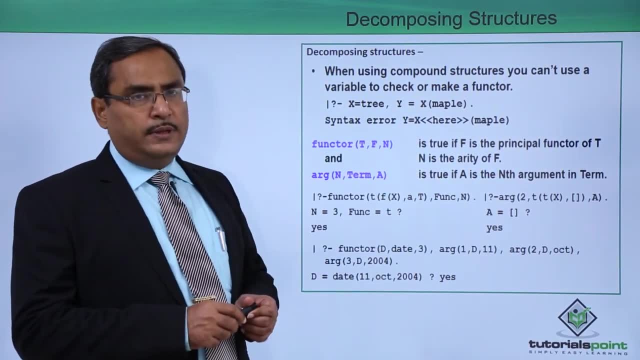 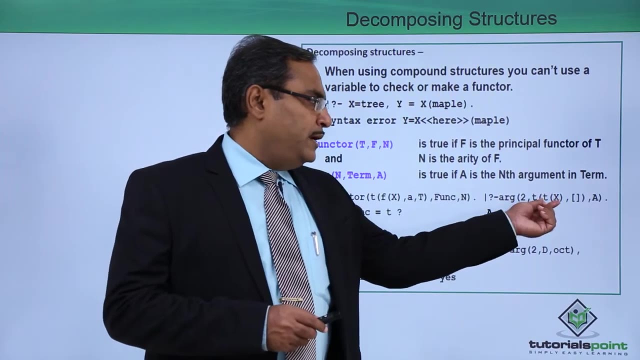 you should do with having this started. So now we are outside of any involved, right? So we need at least this function Now this function. x is the table. why not take this function also? as you have already seen in the program, so this is a very important actually m f's function also. Now here f. 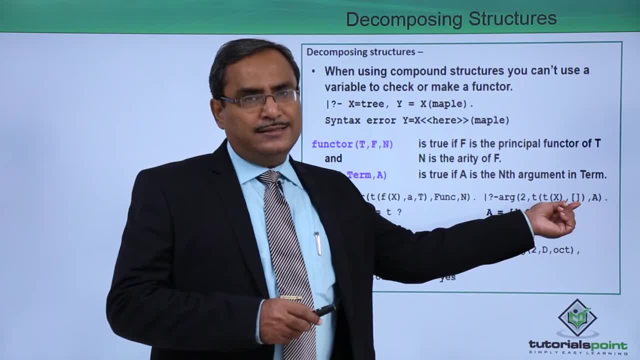 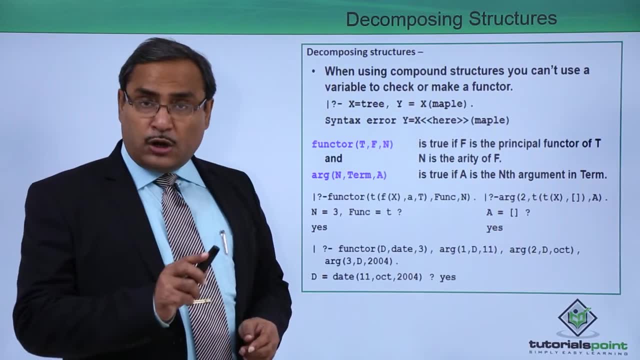 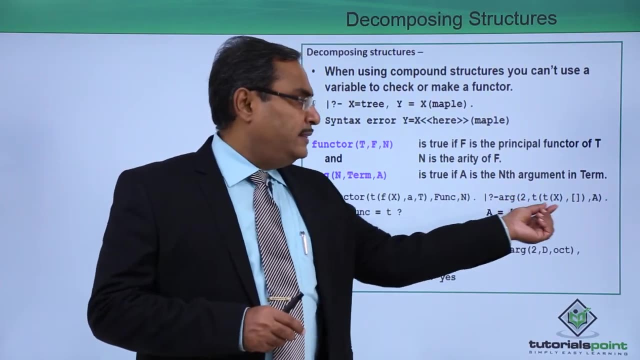 isquarter in here f offensive expression. So this student says, Yeah, find out, or pick up the second argument of this respective functor. So this functor is having two arguments. I am trying to pick up the second one and that is going to be. 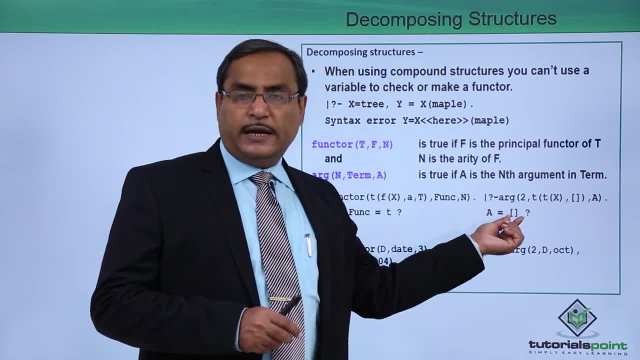 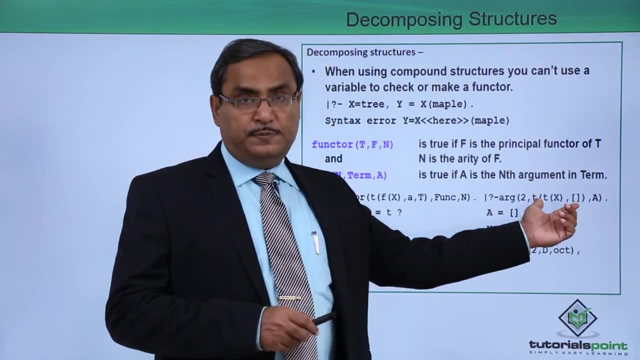 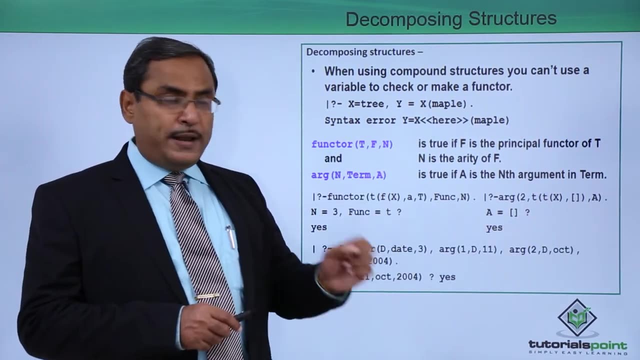 kept in A, So A will be having this third bracket opening, third bracket closing. So that is the purpose of the argument. That means in a respective, in the respective functor. this functor may have multiple arguments, So which argument number you are going to? 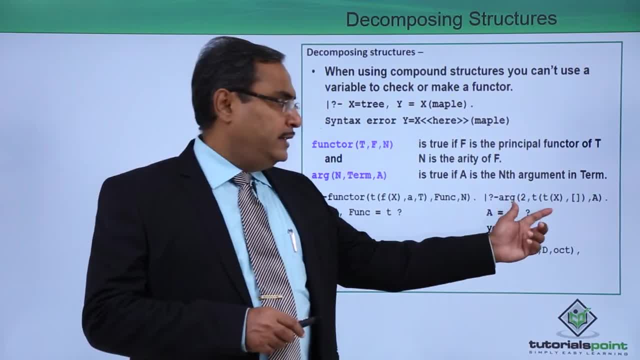 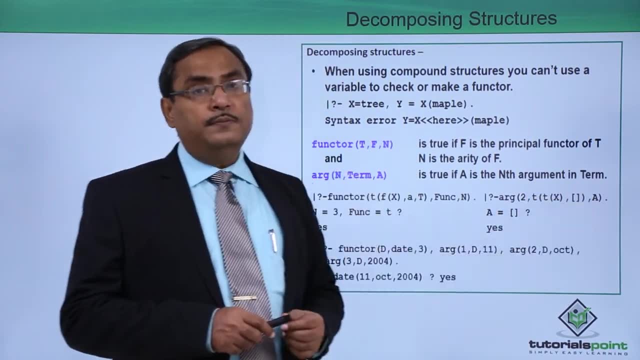 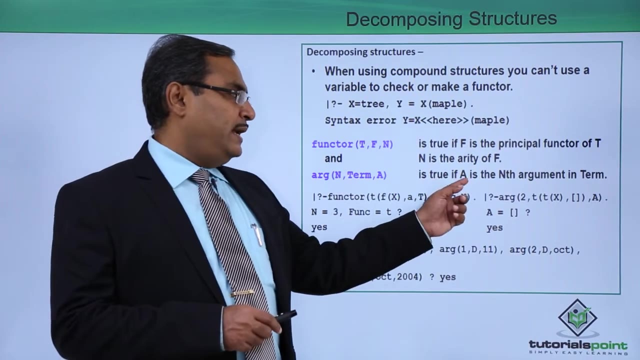 pick up. that has to be mentioned as a first argument and there is a respective declaration, and then in the third argument the respective argument will be initialized. So like this one: So arg n, term A is true if A is the nth argument in term. So that is our issue. 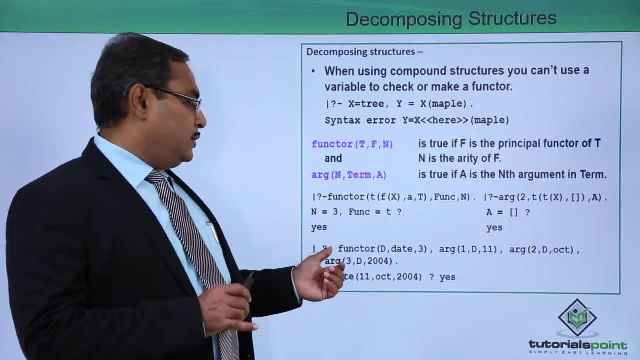 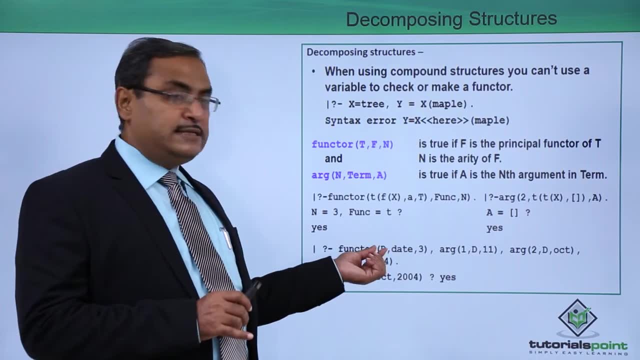 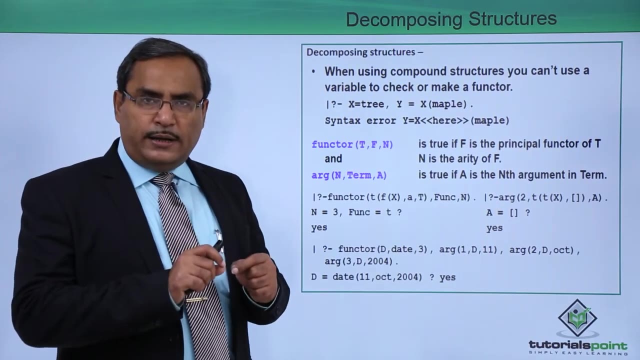 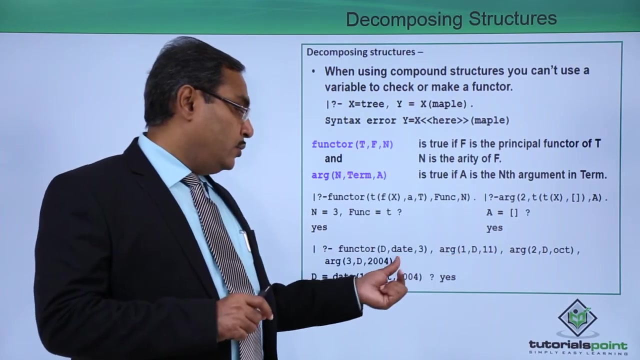 related with this functor and argument. So now it is a very interesting example. just see functor d. So here d is a variable. So argument 1: d, 11.. So you are mentioning that the first argument should be initialized with 11, because here this is a variable. So the first argument: 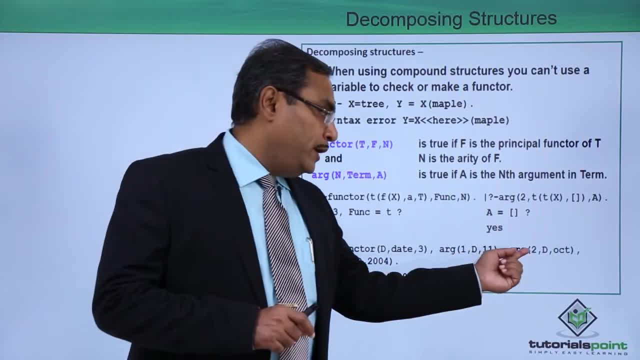 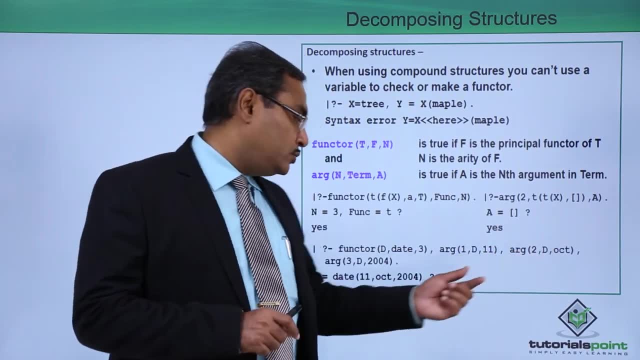 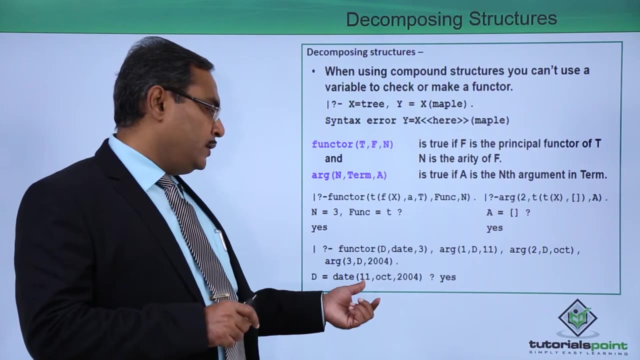 of d should be initialized with 11. argument 2 d oct. So this argument 2 d oct. that means I am putting the second argument as oct, So argument 3 d oct, So al. what is the third argument coming from the last argument that you are putting? 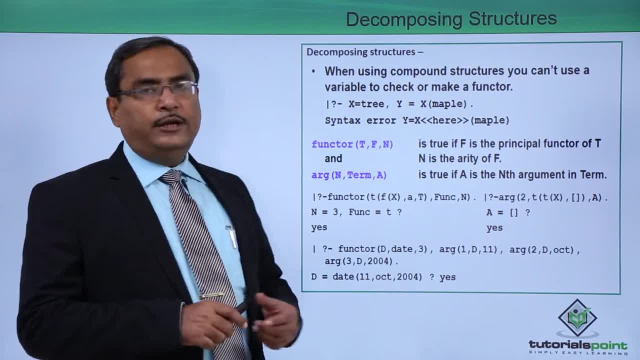 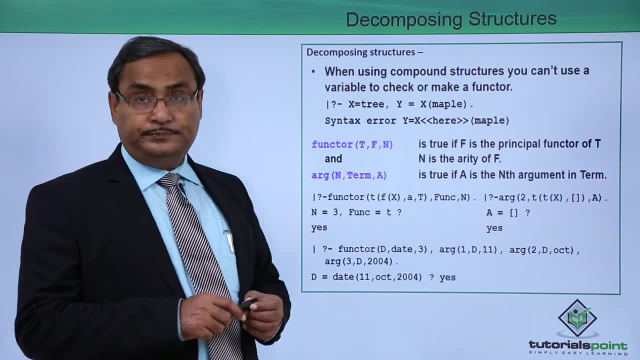 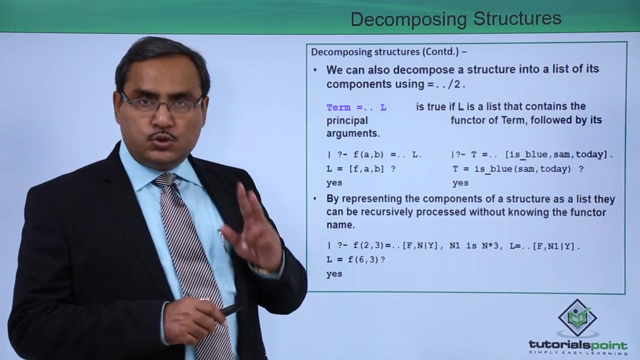 that will beоф S chain 1- 5 and this error will come from the first argument. so this last argument takes the last argument to last argument that may be nth in term. So reflect these in thisществick item. 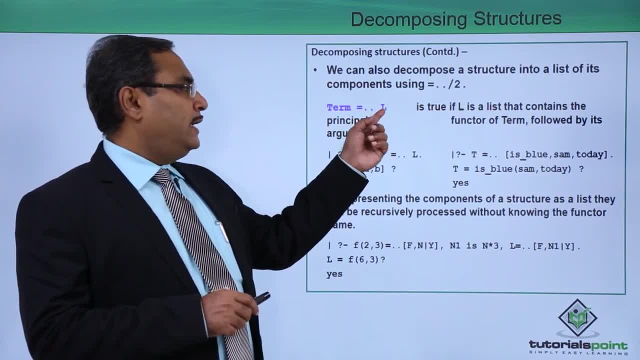 Now the second argument is this: d into the last argument. so this 마지막 argument is eventually the result of returns c, fig. So in this case this was the result. So a result первый, and at the 他 until beginning of the arc was 120.. So a result C, which is: 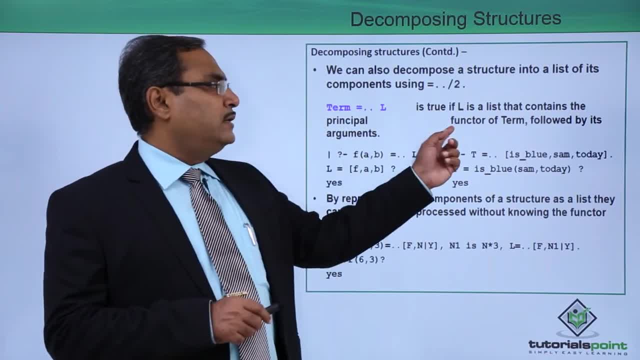 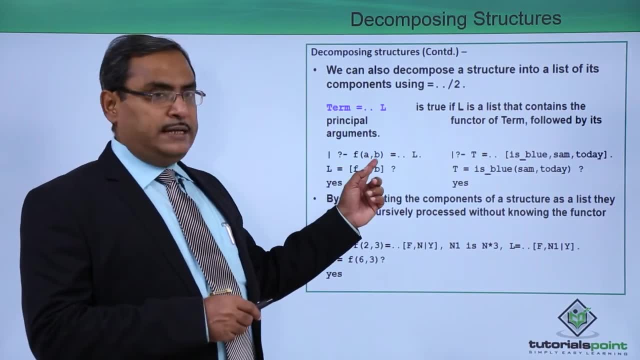 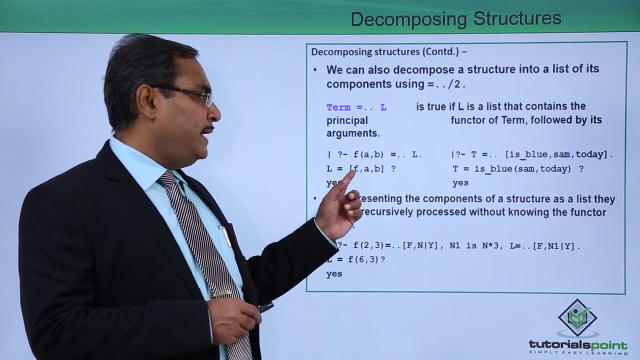 if L is a list that contains the principal functor of term followed by its arguments. So let us go for example: So FAB is equal to dot dot L, in that case this L will be forming this principal functor name and the arguments, all of them in a list. So in this way, this 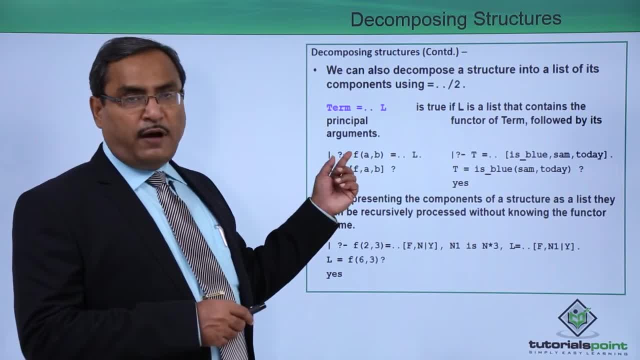 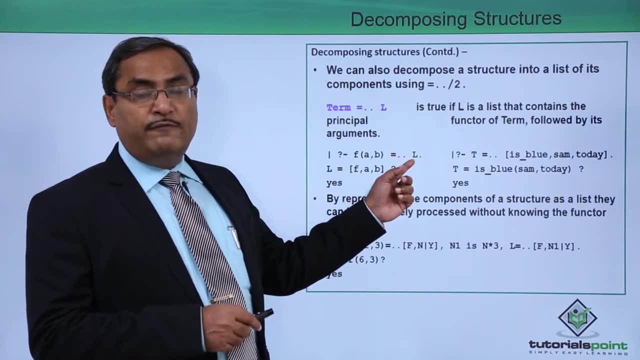 dot dot is working. So that means this is a respective functor name and two input arguments are there? two arguments are there. So if you go for dot dot and if you put one variable name, then against the variable name, the functor name and its arguments will be coming in the 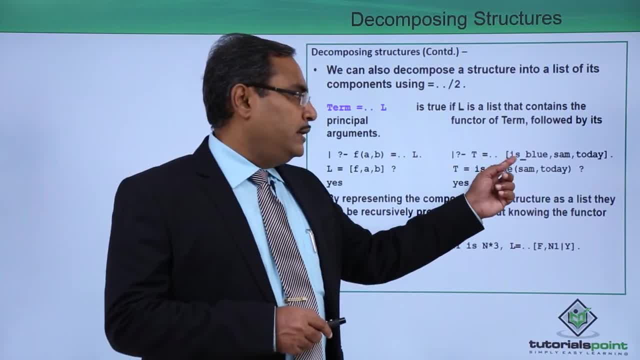 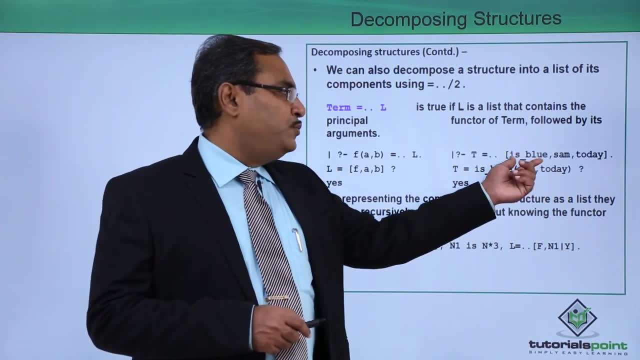 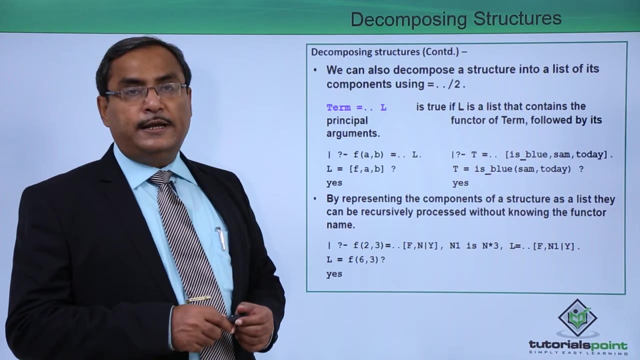 form of a list. So T is equal to dot dot. is blue Sam today. So T is equal to: is blue Sam today. So this is my: is blue will become the functor name. Sam will be the first argument. today will be the second argument. in this way, this dot dot inbuilt predicate is working. 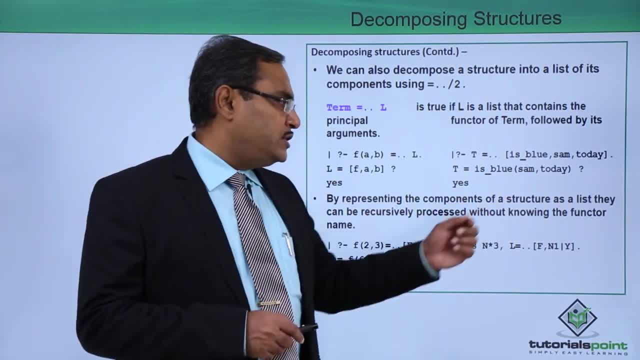 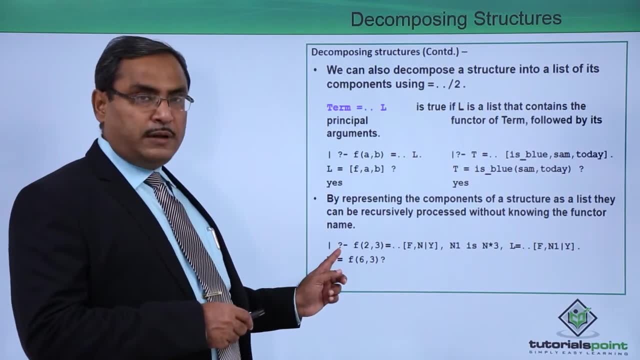 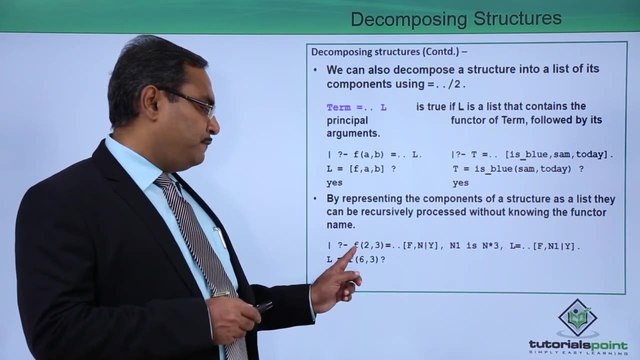 So now, by reporting representing the components of a structure as a list, they can be recursively processed without knowing the functor name. So that means question mark will be there to write the goal: f 2, 3, dot, dot, f, n, y. So f will be coming to initialize this variable, f 2 will. 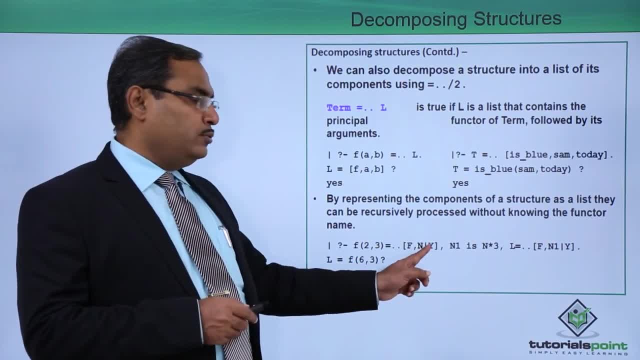 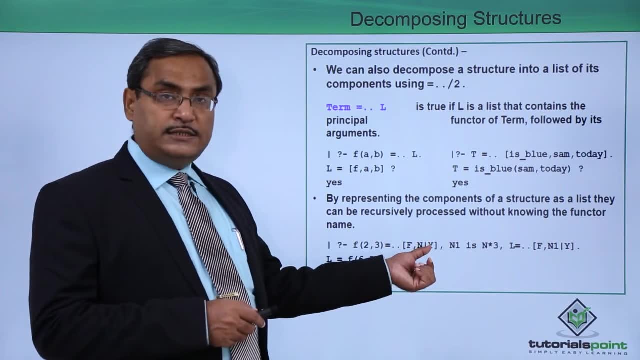 be coming to initialize this. n and 3 will be coming to this variable y. So this list has been expressed in this way: first term comma. second term rest part is tell. So tell will be having 3, n will be having 2 and f will be having the principle functor name. 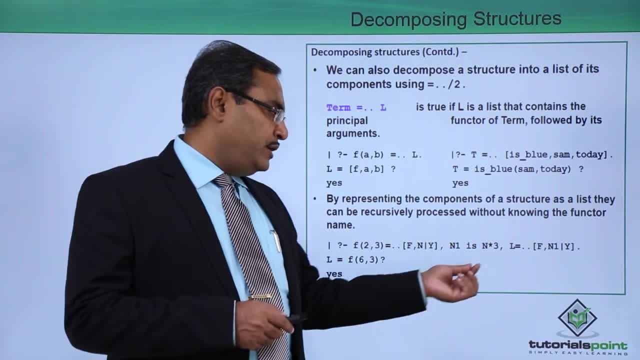 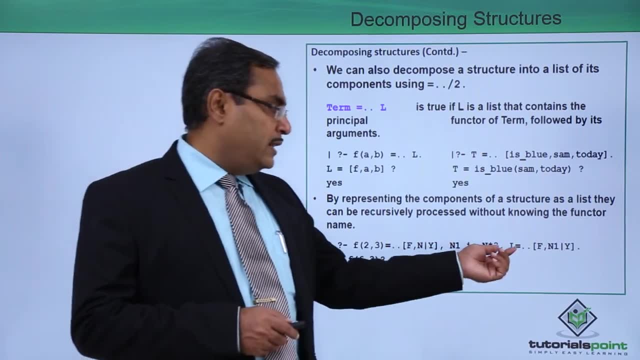 that is f n. 1 is n star 3.. So n is getting 2 here. So n star 3 will be 6.. So n 1 will be 6.. Now we are forming a list that is f, n, 1 y. So f will be our f, because I told. 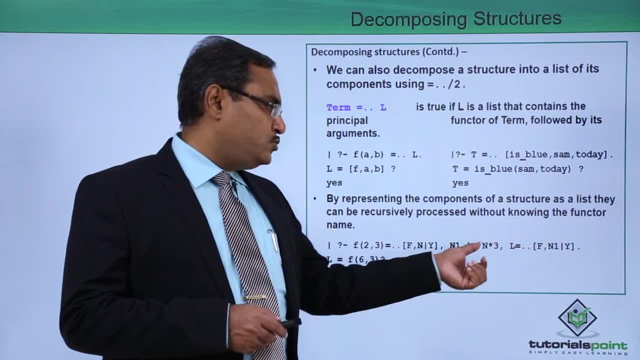 you this one earlier, So f will be our f? n. 1 is 2.. So f will be 2 into 3.. So 6, and here this y is still with this- 3.. So 3 will be coming. 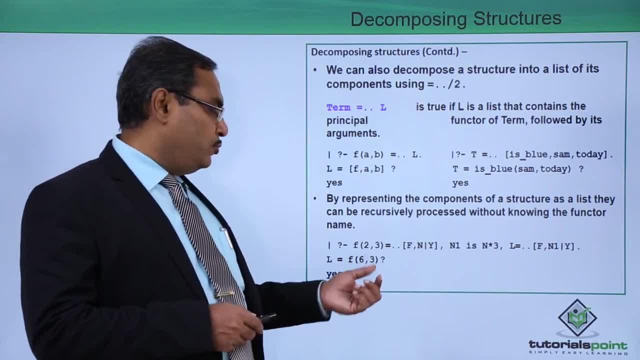 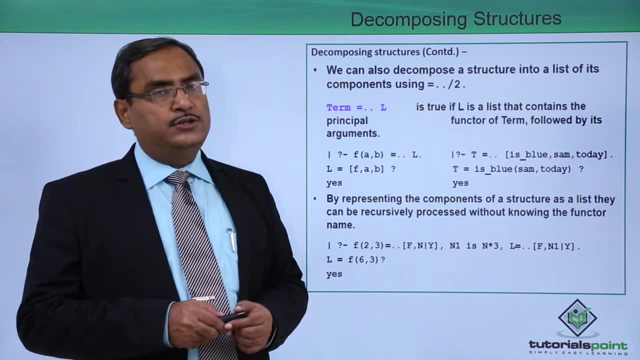 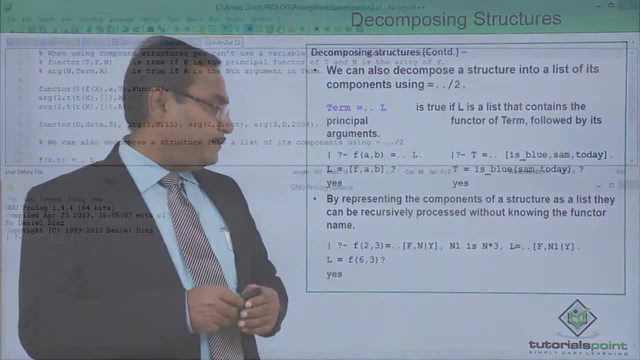 So in this way this respective functor f with two arguments, 6 and 3, will be formed as output. So in this way this dot dot inbuilt predicate is working. So we have discussed different inbuilt predicates with some examples in this session. 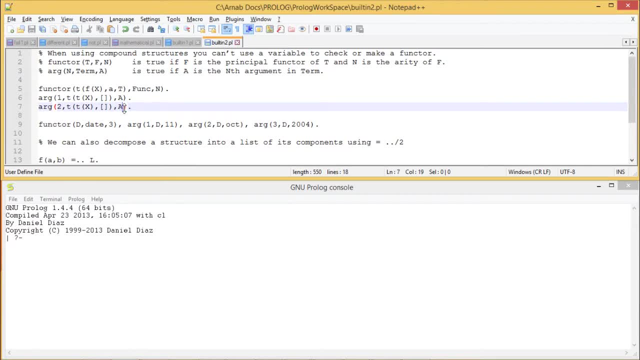 Here at first we are going to discuss our built in predicate functor and ARG argument. Ok, now see when. actually, when we use the compound structures, we cannot use a variable to check or make a functor. So that is why the built in predicate functor is being originated. 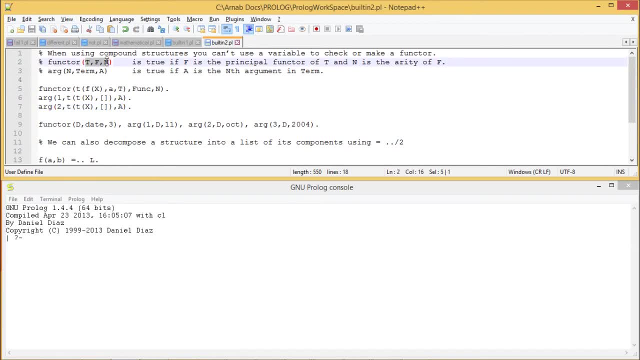 So functor will require 3 arguments, So t, f and n, and this functor will return true. if f is the principle functor of capital, T and n is the addit, That means the number of attributes or number of arguments of f. 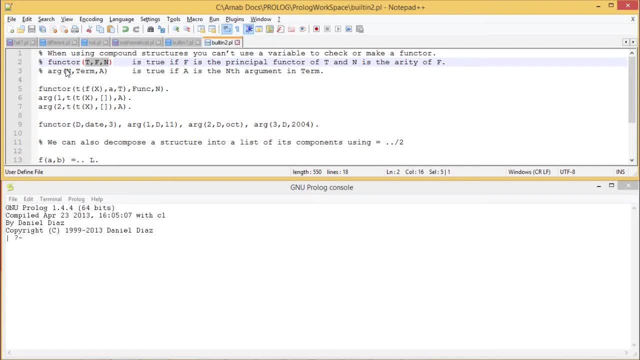 And argument that is ARG. this very predicate will have 3 input arguments, So n term and a will be returning true if a is the nth argument in the term. Ok, now let us go for some practical demonstration for the better understanding. So here in. 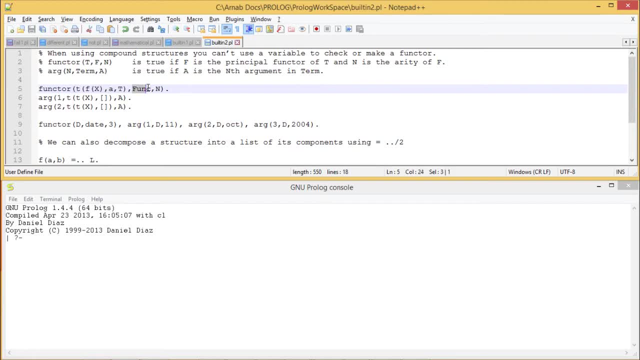 this case. this is my first argument, this is my second argument and this is my third argument. Ok, so n will be returning the number of arguments here. So that means here we are having number of arguments is equal to 3.. So, first, one second, one third, one fourth. 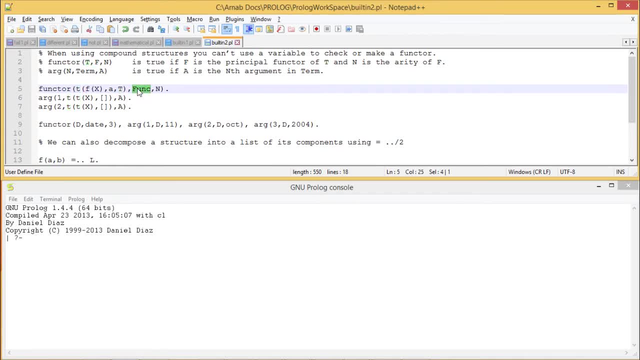 one, fifth one, sixth one, seventh one and the third one, And this functor, this particular variable, as it is starting with the capital letter, will be returning the respective functor name. So let me execute the code at first. So I am just making a copy and executing this. 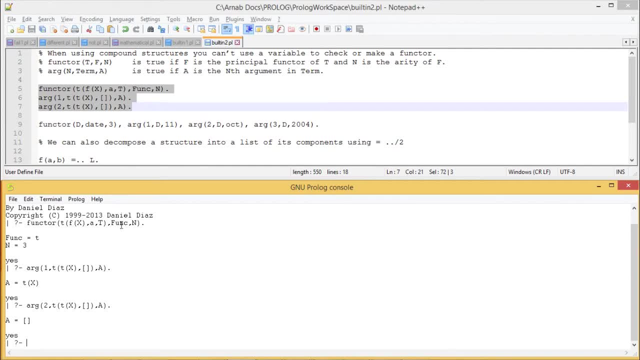 one. So now, here you see, I have executed this. So functor is get got initialized with t. that is the functor name and n is the number of arguments, as I told you that it is having three arguments. So that is why n is equal to 3 here. Ok, 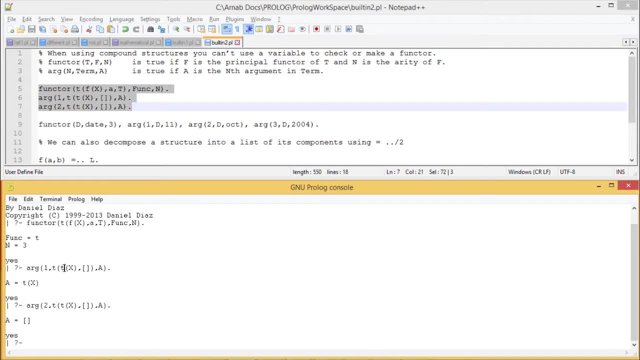 Now see, this is the functor name and it is having two arguments. So one is this tx and this third brackets md. So now, if we want to retrieve the first argument in the variable a, so I must be getting this tx. So if I want to retrieve the second argument of this, 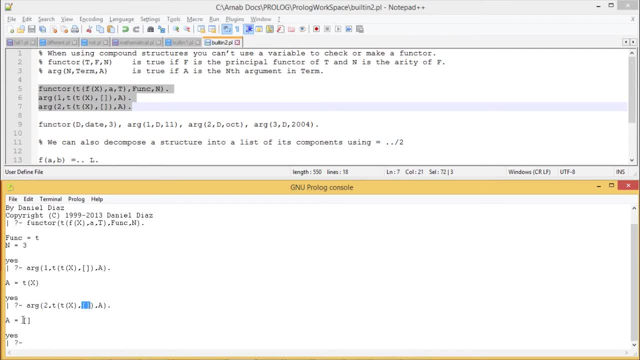 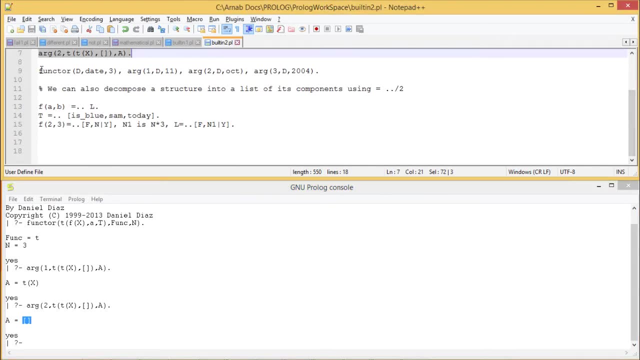 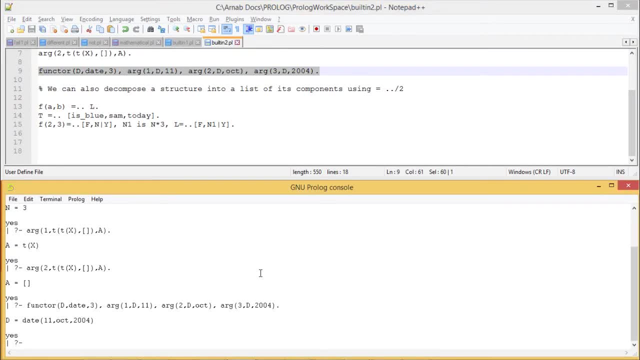 execution. If I go for this execution, you can find that functor d date 3.. So here we are expecting three arguments. The first argument of the functor d has been initialized by 11.. In this way, second argument of d has been initialized by october. In this way, that is. 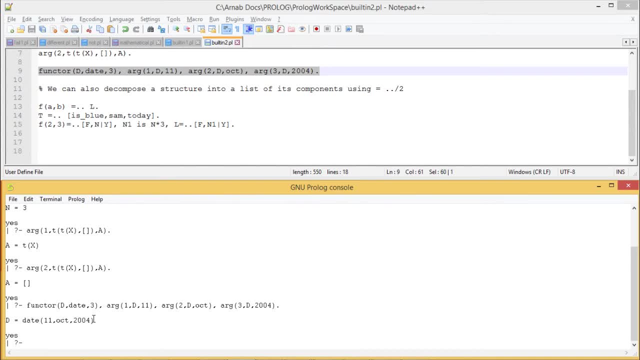 2004.. And you are getting this one that it is having the respective outputs as well. So d is equal to date within bracket 11, comma october, comma 2004.. In this way, we are getting this output. so now we are going to have a very interesting one, that is, a dot dot. so now, what is the purpose? 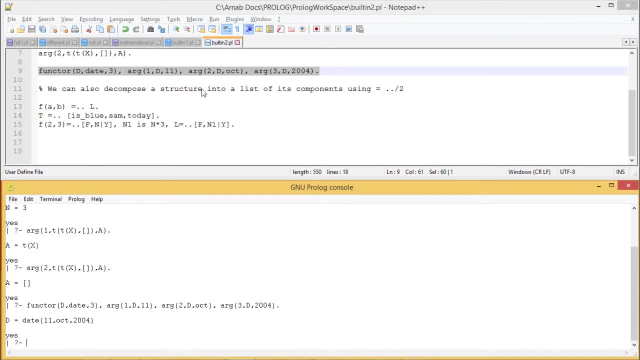 of this dot dot. actually, we can decompose a structure into a list of its components using this dot dot. okay, now how this code is getting executed and what is the respective meaning of this dot dot. let me explain that one into details. okay, now see here. this is a respective functor. 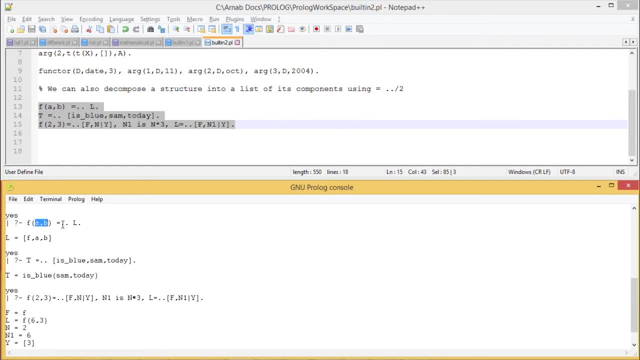 and it is having two arguments. i'm converting it to a list. i'm converting it to a list, so now what will happen? so this functor name and these two arguments will form one list. i can have other arguments also. it is not mandatory that i shall be having only two arguments in this functor i. 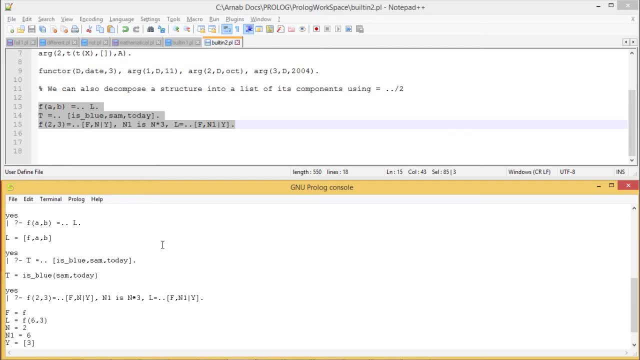 can have multiple arguments and they will be working fine as well. so now let me show you that one also. so if i go for this and if i make this one, as if i make this one as, say, say, cdef, in this way also, it will be giving us the respective outputs. okay now. 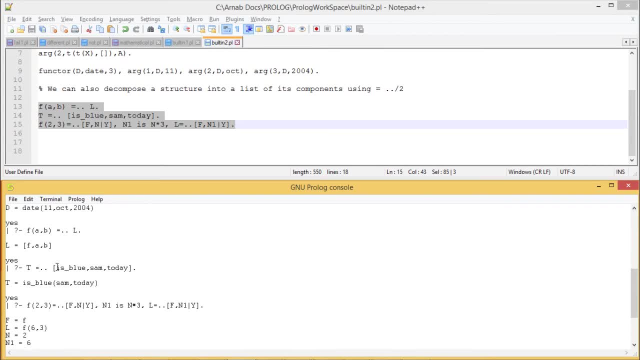 t we are having is equal to dot, dot, and this is the list we are having. so the first one will be the functor name and other two will become the attributes. so accordingly the t has got initialized accordingly here. also i can put other arguments and they will be coming in. 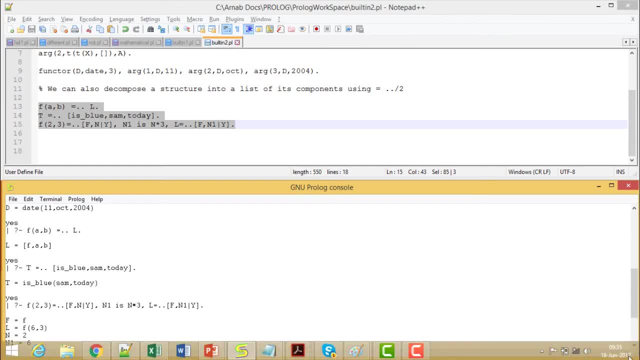 this argument list as well. so now let me explain this one. let me explain this one. now what is happening? you see, f is equal to. we are having this one as f 2 comma 3 is equal to dot dot. so this is the respective expression. we have written the query. we have written the goal. 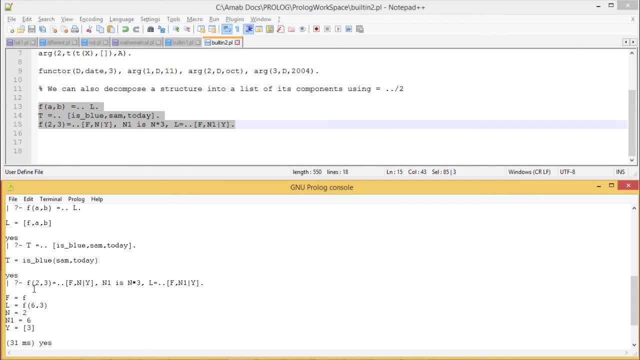 we have written, so now let me explain it. so here you see, this is my f, that is the functor name. this is the first argument. this is the second argument. so here this f, so the first. so when it will get form a list, so the first element of the list will be the functor name. so that's why it is having this. 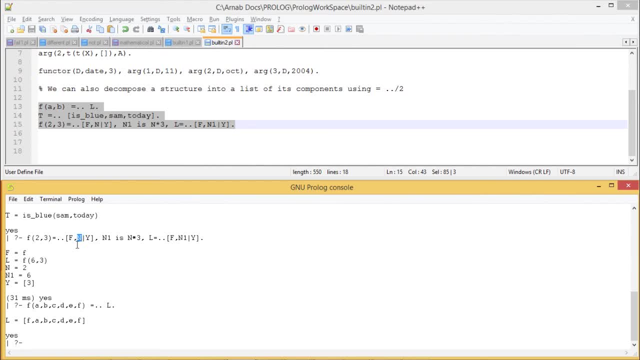 f here. okay, now, now this. now we are having this, the second argument. so we have divided this one as the head and tail. so head will be 2 here as well. so n will be initialized with 2 and y that is a tail part and that will be the least containing 3 only. so y will be the least containing 3 only.